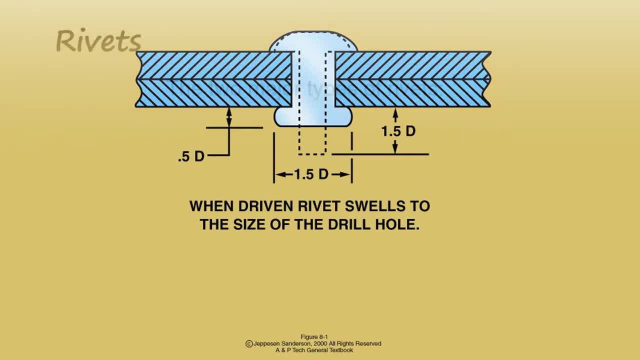 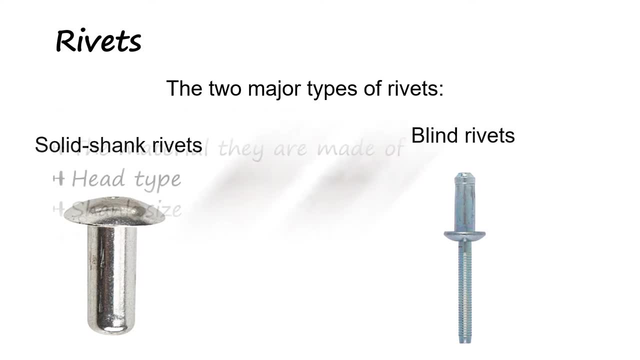 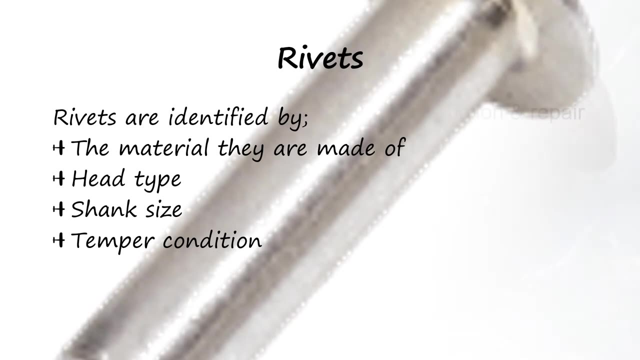 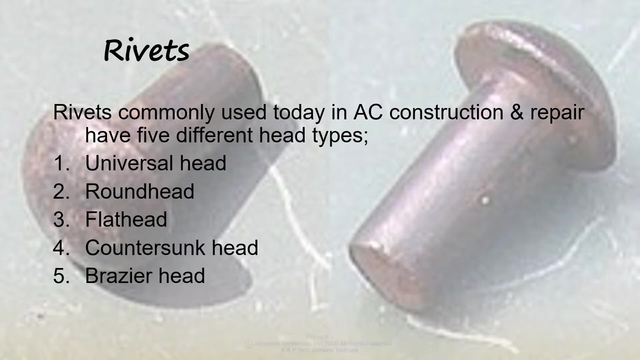 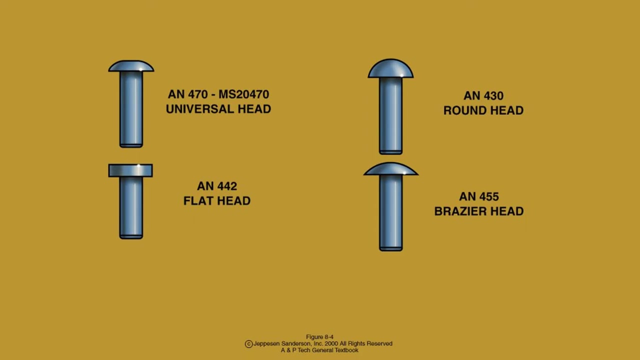 of the shank. For quiz purposes, you will want to memorize the 8n numbers for these rivet head shapes, as well as the number of rivets held to the top, the weight of the shank and the number of rivets held to the bottom. 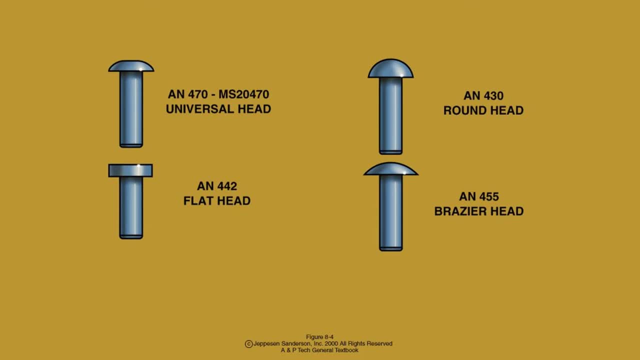 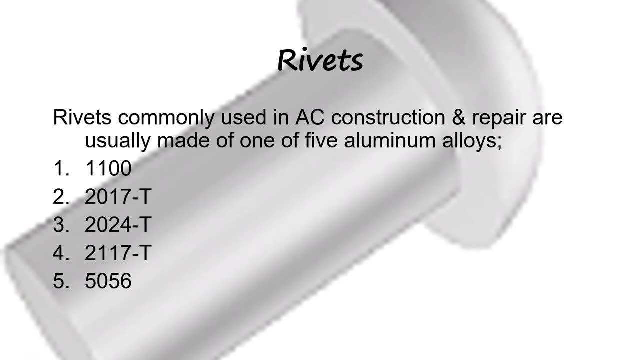 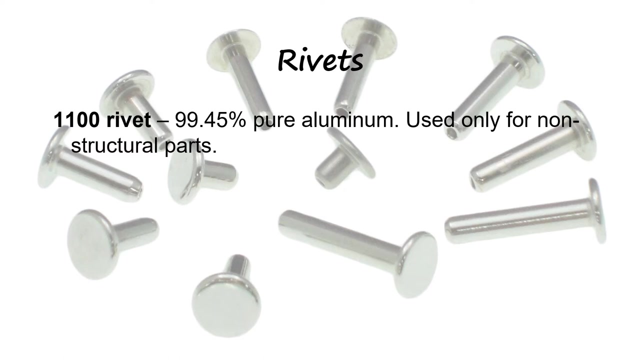 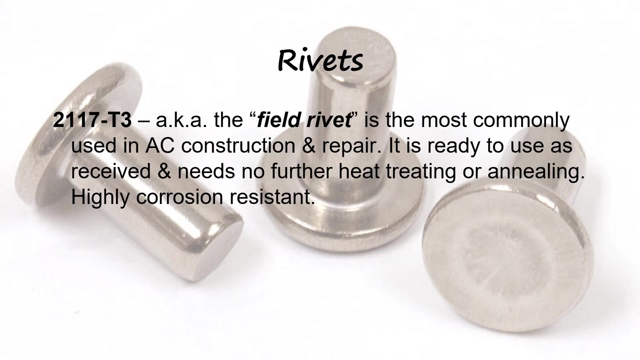 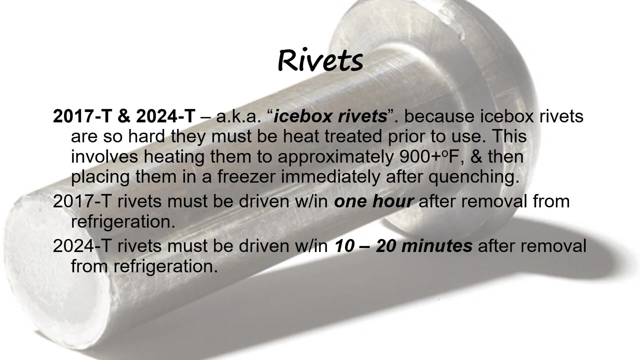 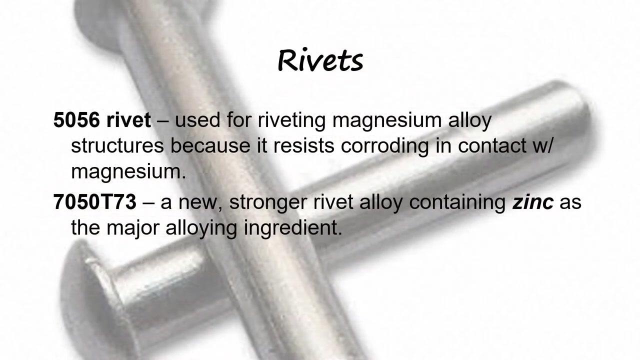 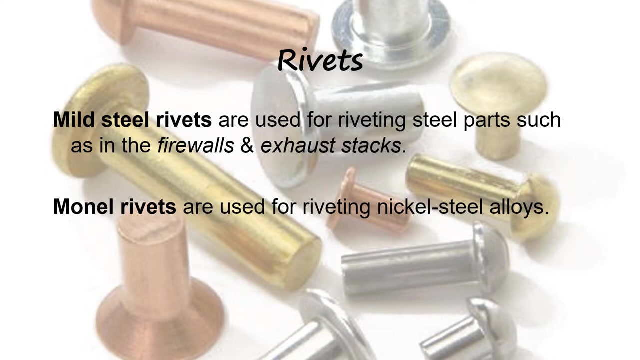 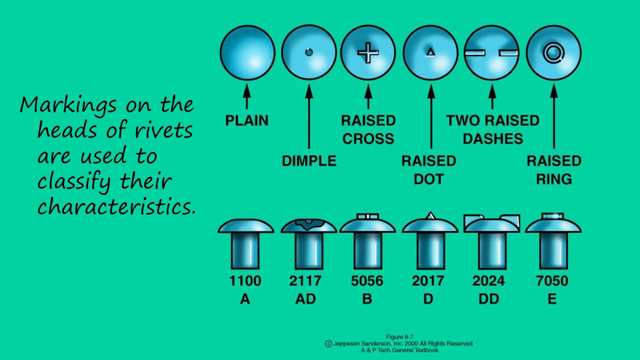 For quiz purposes you will want to memorize the 8n numbers for these rivet head shapes, the name of the head shape. You should memorize these rivet alloy numbers and corresponding one or two letter alloy identifiers and the rivet head markings they correspond to for quiz purposes. 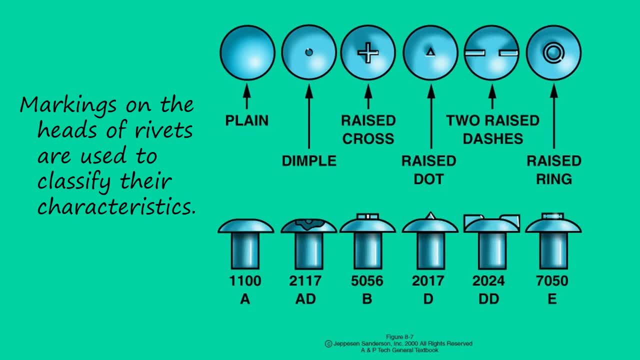 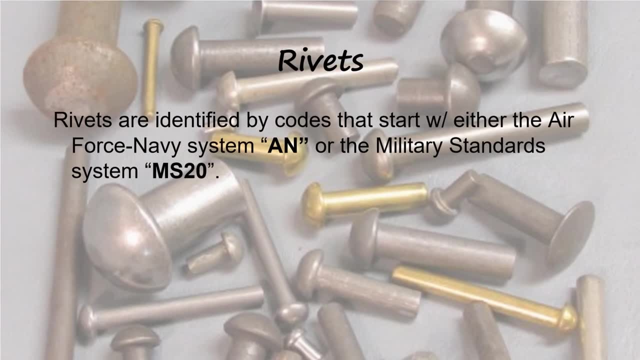 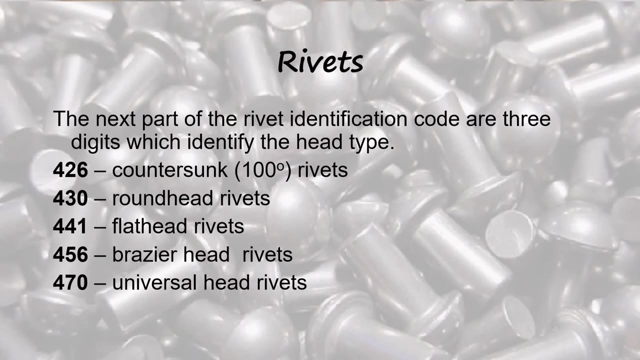 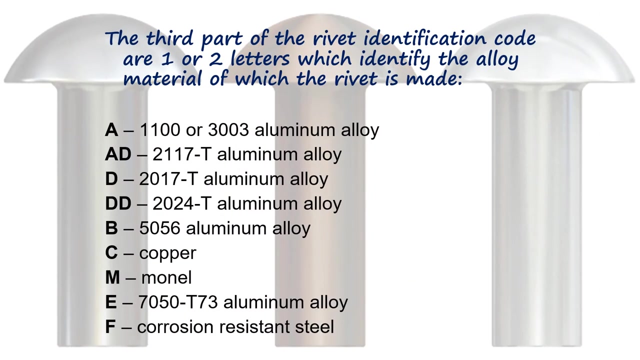 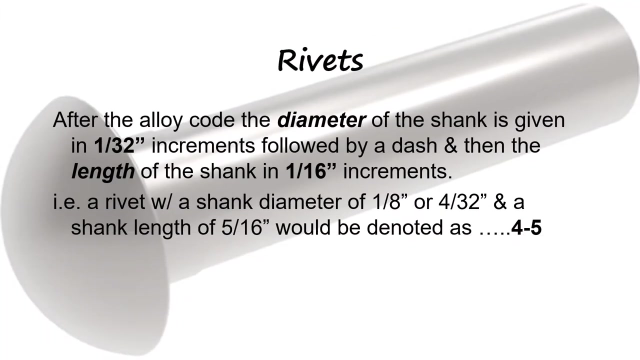 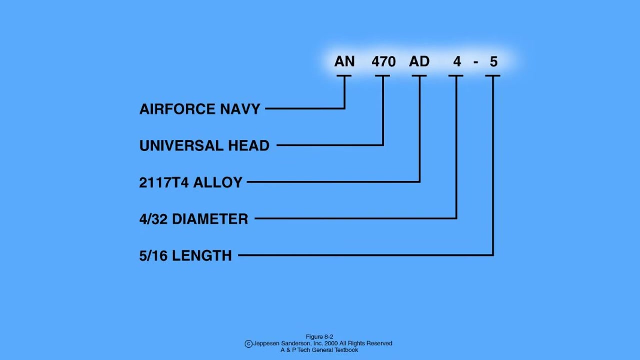 Now let's go ahead and take a look at some of the things that you can do to determine which one is the best fit for you. Now we can see how the part number for a rivet fully describes the rivet. In the part number AN470AD4-5,, the AN gives us the standards the rivet was built to. 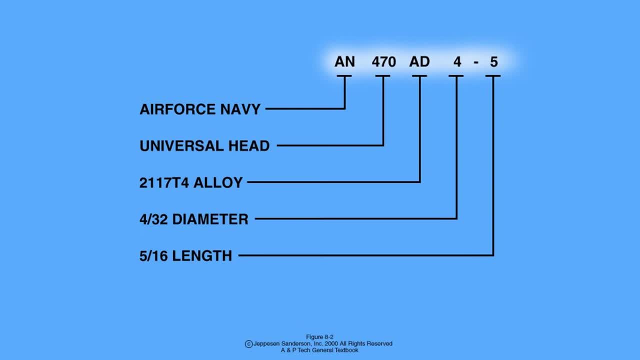 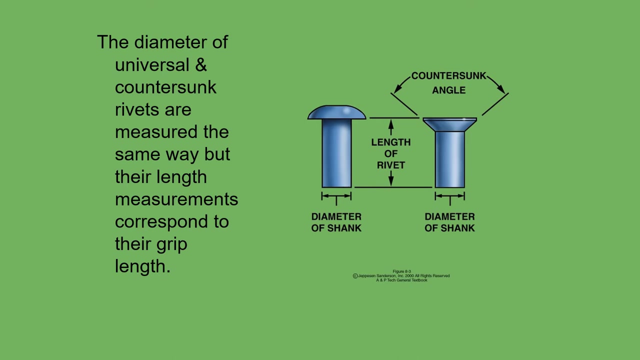 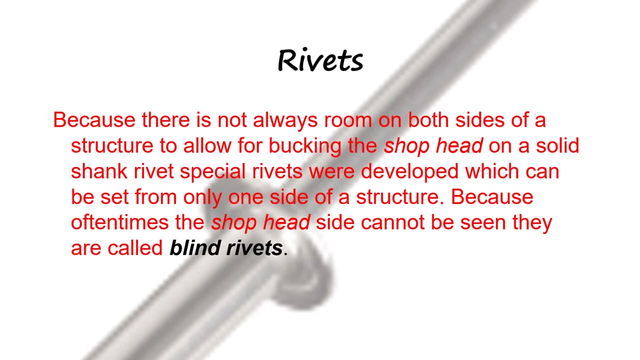 The 470 informs us of the shape of the rivet head, The AD informs us of what alloy the rivet was made of and what heat treatments it has undergone. And the 4-5 tells us the diameter and length of the rivet shank.